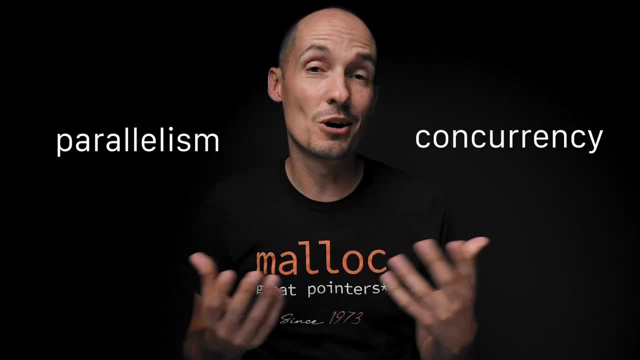 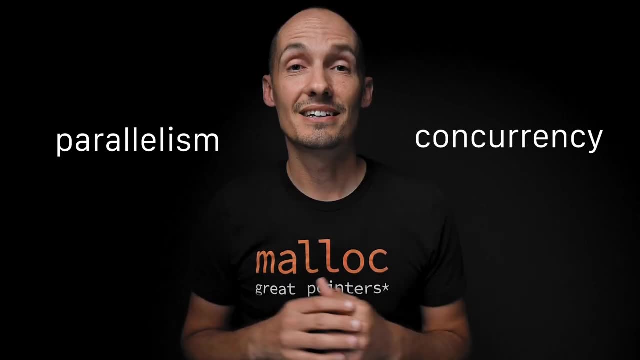 But today I wanted to talk about them, just to try to make your lives a little easier and help you sort them out, to try to bring a little more precision into our discourse when we're talking about software and how our programs work. Also, different people's definitions on these terms. 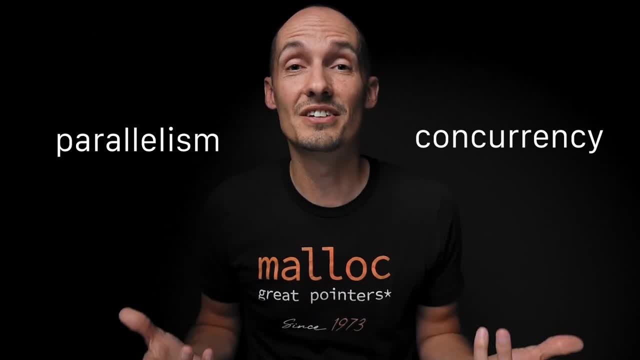 may vary slightly. I'm going with mine and what I've seen in the field and what seems to be typical, but if your operating systems professor happens to have a different opinion on what you're talking about, then you're probably going to want to talk about. 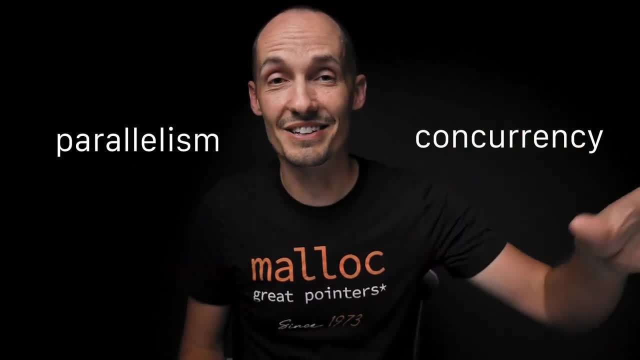 a different set of definitions, Please go with theirs, and at least until the class is over. And then, of course, you can tell them they're wrong. So what is the difference? Well, let's start with the idea of parallelism. So parallelism. 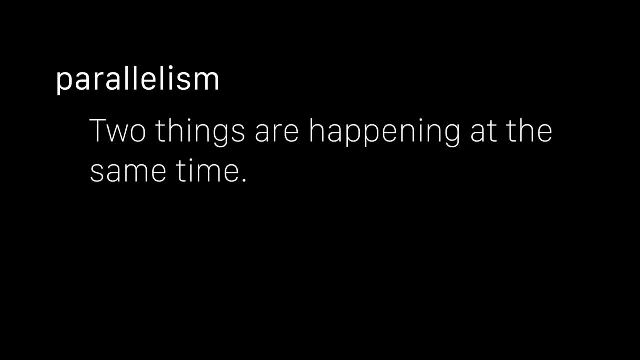 simply put, means that there are two things happening at the same time. Okay, so sometimes we think about parallel computation. that would mean that two computations are occurring at the same instant in time. Now, typically this requires some kind of hardware support, right? So this: 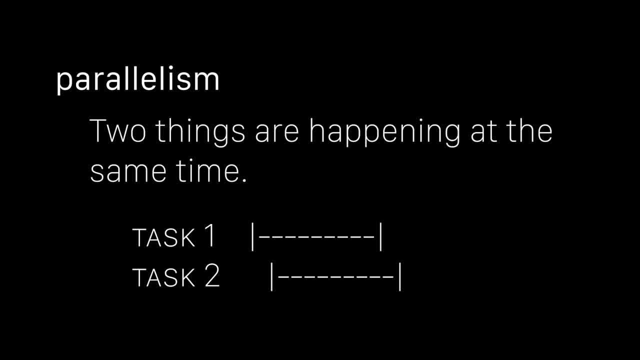 could be two tasks that are being executed simultaneously on two different cores. right, They're happening at the same time. So literally you could have two things happening at the same instant in time. and if I take two tasks, let's say each task takes a second and 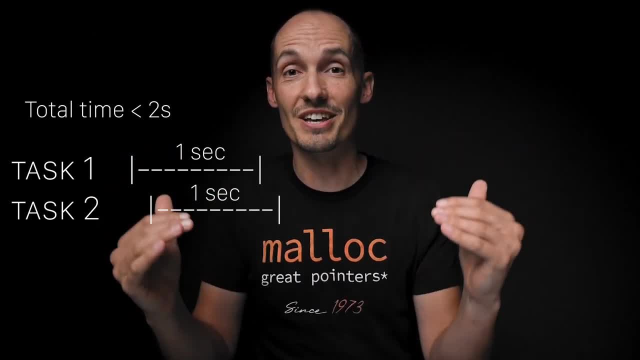 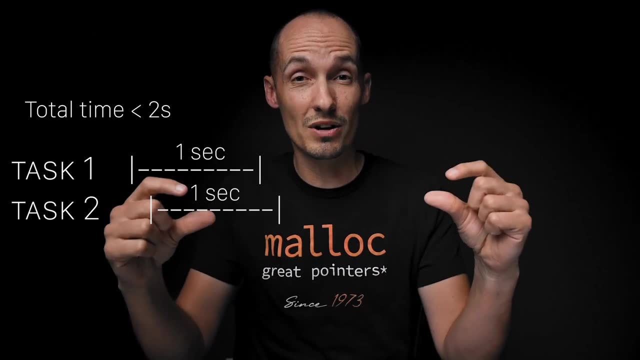 I run them in parallel. I should get them done more quickly because they're actually happening at the same time as long as they don't depend on one another. But if they depend on one another, then they're not going to be really done in parallel because one of them is going to have. 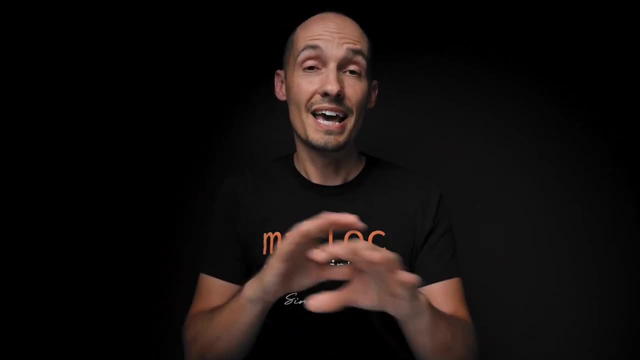 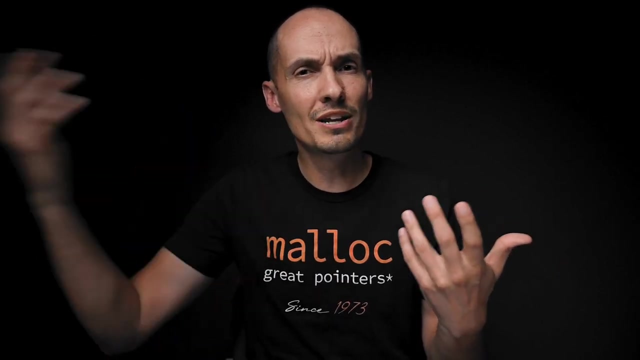 to wait while the other one finishes. Okay, so parallelism means computation is happening at the same time, and this isn't just about processor tasks. This could also be two different operating operations, like reading from a disk. The disk may be servicing a read request while I'm doing. 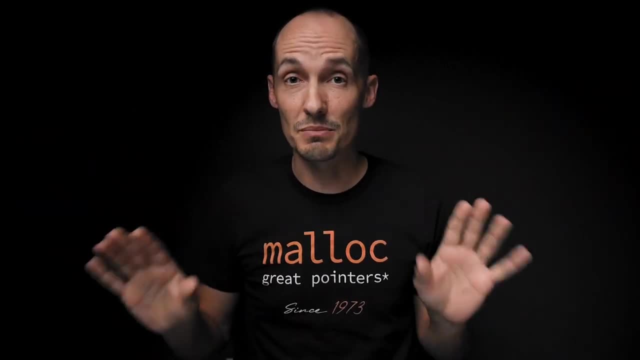 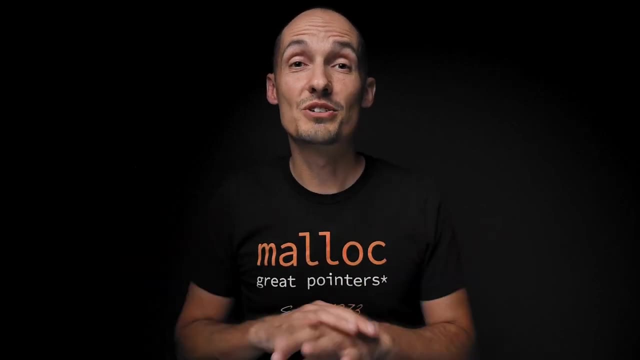 computational tasks, and those two things could be happening at the same time because they depend on two different pieces of hardware that are each able to work independently of each other. Also, of course, you can have computation being done on separate machines, separate servers. You see this. 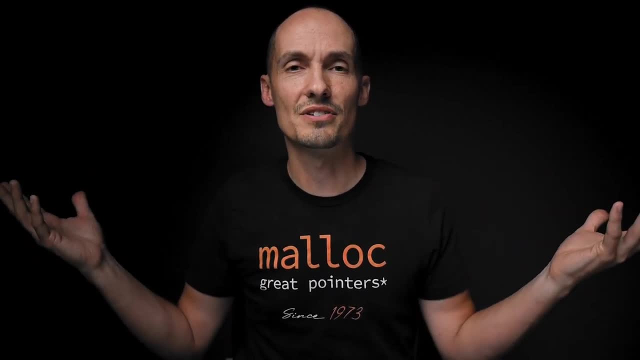 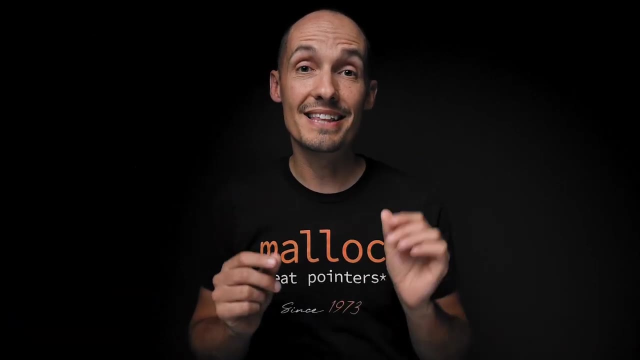 a lot in big supercomputers, compute clusters that have many processors. So yeah, multiple cores, multiple processors, it's all parallel. Now, concurrent is a little different. If two tasks are concurrent, that means that they start and end at the same time. So if you have two tasks,